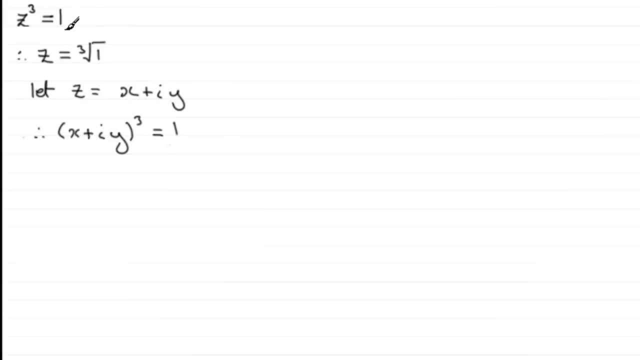 is how we can go about finding the nth roots of 1.. And I'm going to use the example Z cubed equals 1 to demonstrate this. But the method would equally apply to any other roots of 1.. Now if we were to take a complex number, Z, and write it in mod arg, for Z we'd have to 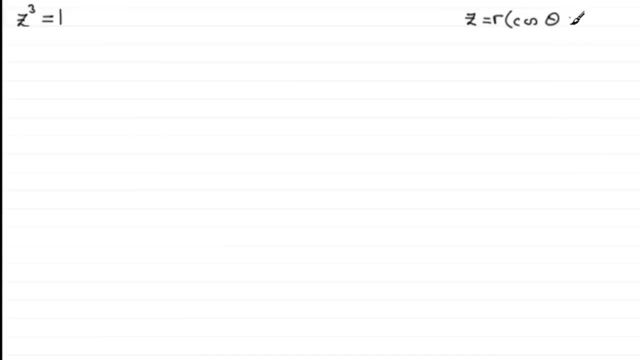 write it in exponential form, In other words r cos theta plus i sine theta. Or you could write it in exponential form: That would be r e to the i theta. Now suppose I was to represent the real number 1 on an argon diagram. If I was to draw my 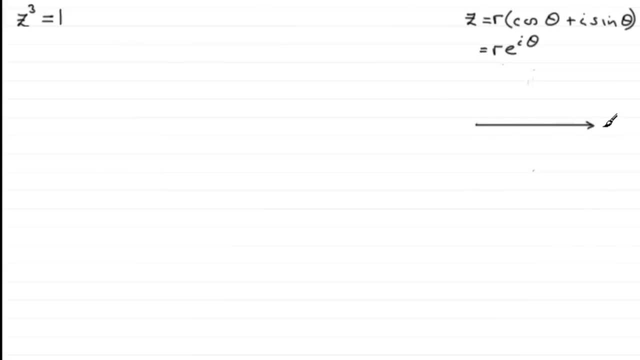 axis. let's say we have a real axis, something like this, And we'll take our imaginary axis, We'll come down here, So that's our imaginary axis. Then the real number 1 would be represented something like this: We'll have that, Put an arrow on there And that would go to 1 there. 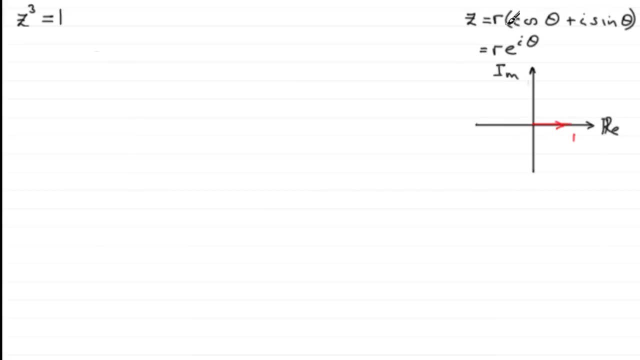 So if I was to represent 1 in this particular form here, r would be 1.. The arg of theta. well, that would be 0 radians. So I could just write r cos theta plus i sine theta. write one here as being the cosine of zero radians plus i sine zero radians. 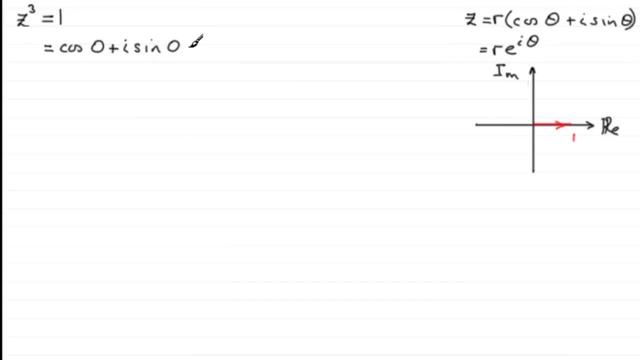 now, okay, i've got it in this form, but i could add any multiple of two pi to the arg and i would still get the same result. it would still come to one. so what we do is we rewrite this as the cosine of 0 plus, say, 2k pi where k is an integer, and for the imaginary part i write it as i sine of 0 plus. 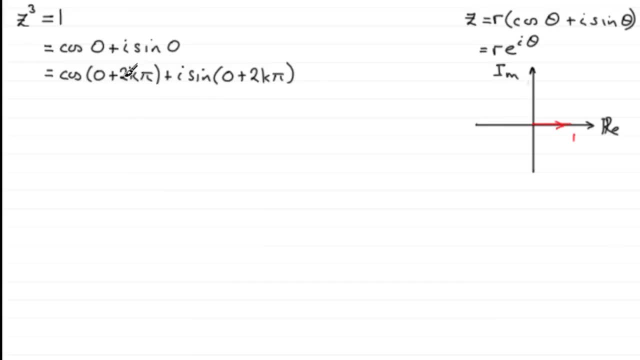 2k pi. okay, so hopefully you got the 2k pi bit, okay, OK, it's just saying that we could go from here and do any multiple of 2 pi and it will keep bringing us back to this particular place. OK, well, we could simplify this. We don't need that zero anymore. 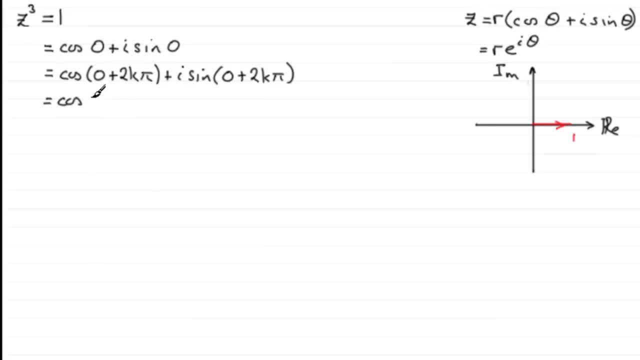 So we could just write this then as the cosine of 2k pi radians plus i sine of 2k pi radians. Now, if we use DeMarva's theorem, OK, we know that z would be equal to the cube root of 1.. 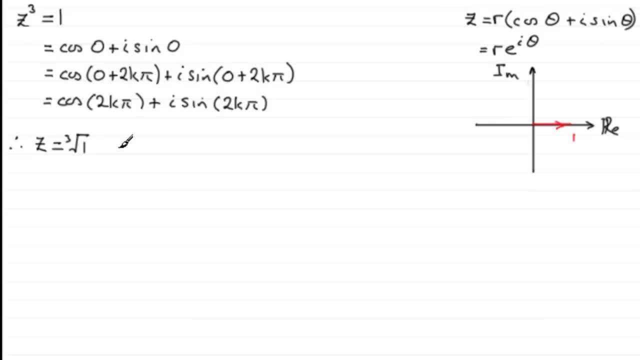 All right, And in other words, that's going to be 1 to the power, one third. So we've got to write all of this then to the power- third. So what we've got then is that this is equal to the cosine. 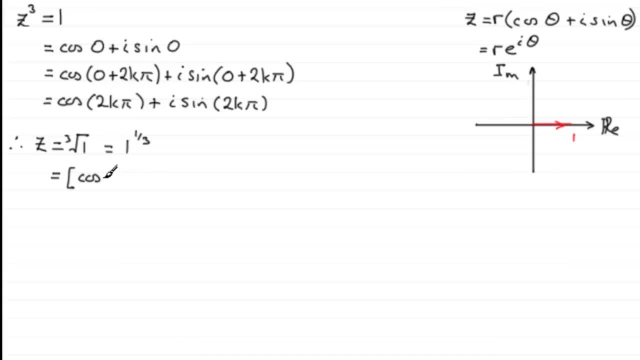 Let's put some square brackets there, The cosine of 2k pi plus i sine 2k pi, And all of this lot is raised to the power one third. Now by DeMarva's theorem we know that we can bring this power down to the arg. 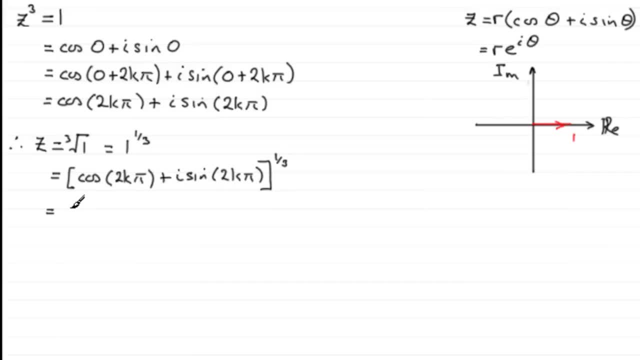 We can multiply it with the arg here. So in other words, what we get is the Cosine of 2k pi over 3.. And for this result it'll be i sine of 2k pi over 3.. Now I've used the mod arg form to get to this result here. 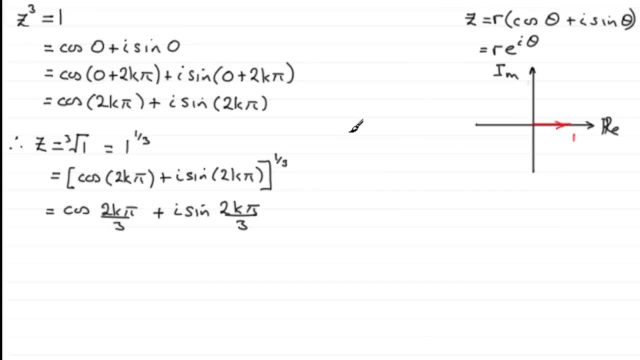 You might not want to use the mod arg form. There's other ways that you could do this. You could use the exponential form. So I'll just quickly bring you up to speed on that, because it will change from one textbook to the other or from one teacher to the other. 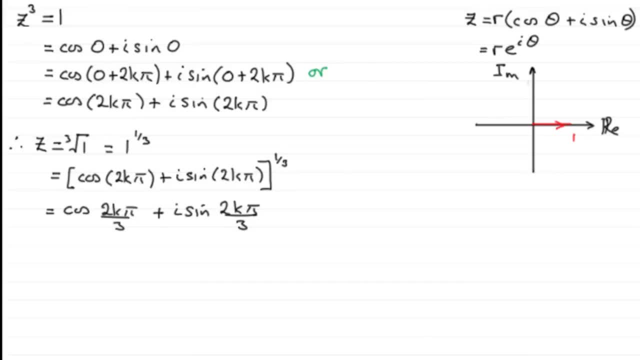 So we'll have a different method. If I was to use the exponential form, then in place of this result here for z cubed- let's just put down we've got z cubed would equal R. R is the modulus, which is 1.. 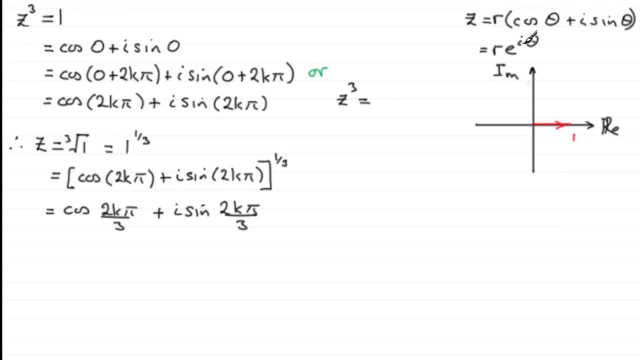 Okay, So we've just got one. We can leave that off, And then it'll be e to the power i. And then for theta: theta is the arg. We can represent it as 2k pi. So just put that in brackets: 2k pi. 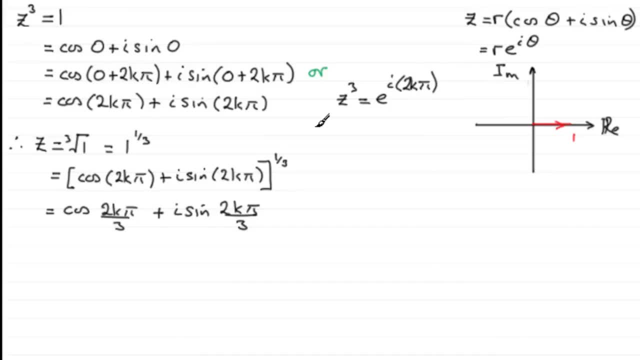 All right. So when we take the cube root we've got: this is now raised to the power of third. So what we've got is therefore: Z would equal- and we'll put this in square brackets here- it would be- e- to the power i 2k pi. 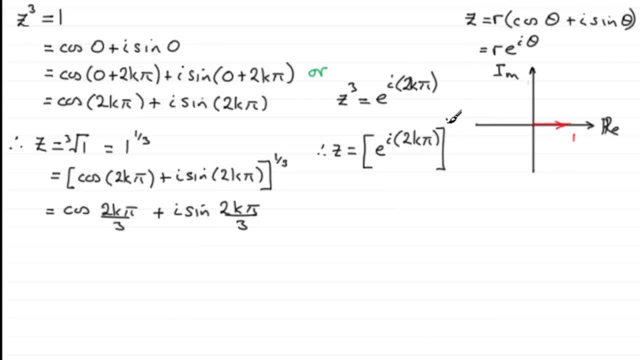 And all of this would be to the power one third. And if I'm doing something like this with powers, then I just multiply the power by the third And what we end up with is an equivalent statement to what we've got here, That is, that z equals e to the power, i, 2k pi over three. 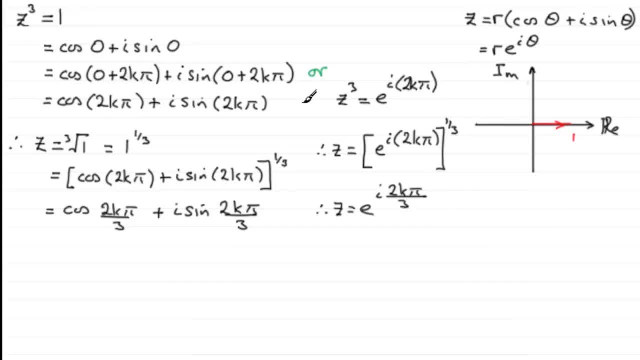 Okay, So we've got the mod arg form or the exponential form. It's totally up to you which version you want to work with. So where do we go from here? Well, we know that when k equals zero, let's just write it down here. 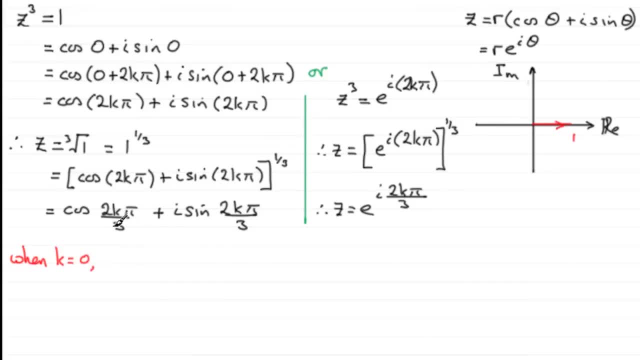 When k equals zero, we end up with the cosine of zero plus i sine zero, In other words what we had up here, which is one, This result here on the argon diagram. So we'll just write then that z equals one. 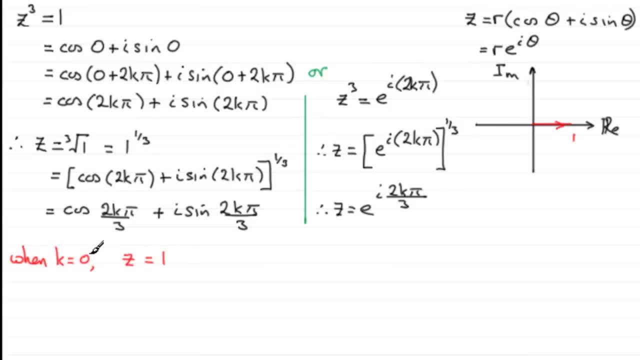 Now suppose we take another integer value for k, Let's say when k equals One. Okay, Now when k equals one, what do we have this time? Well, z would be equal to the cosine of two pi over three or two thirds pi. 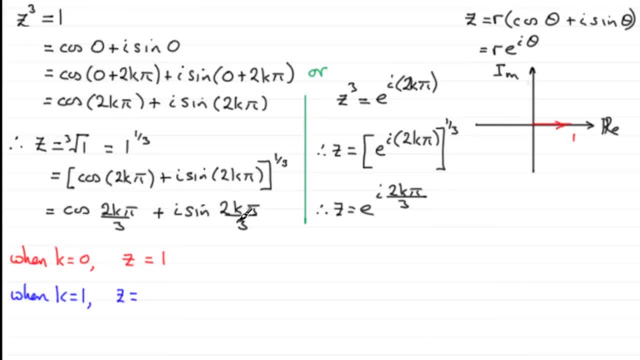 And here we'd have plus i sine of two thirds pi. So let's just write that in: We've got the cosine of two pi over three, two thirds pi, Plus i sine again of two thirds pi. Now what does this result in? 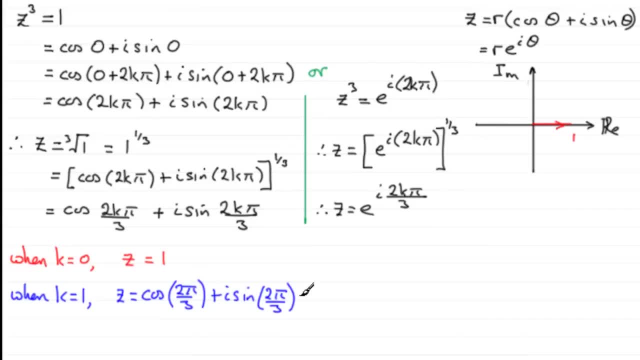 Well, the cosine of two thirds pi is minus a half, So we get minus a half. And then the sine of two pi over three. two thirds pi is positive root three over two, So we've got plus i. And then the sine of two pi over three. two thirds pi is positive root three over two. 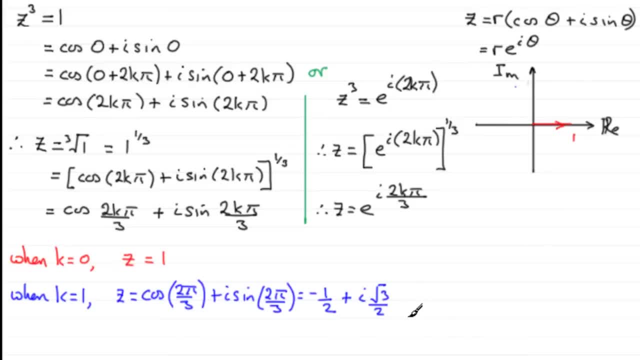 And we could represent this on our argon diagram. We've got that. the argon is two thirds pi and the modulus is one, So it's going to look something like this: I'll just put an arrow on that one, Okay. 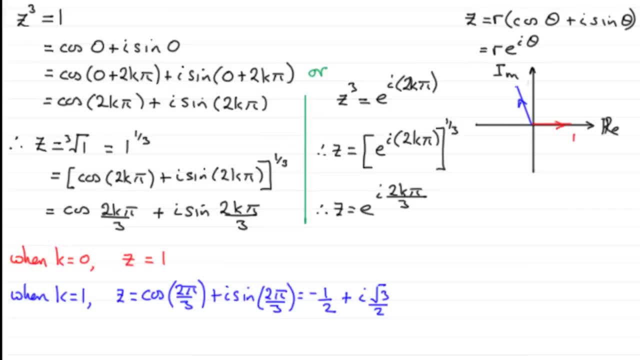 Now what happens if I put say k equals two through here. Well, what happens if I put say k equals two through here? Well, I get the cosine of four thirds pi plus i sine four thirds pi. Well, I get the cosine of four thirds pi plus i sine four thirds pi. 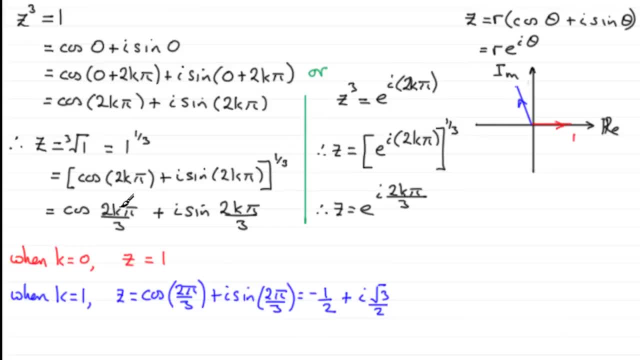 But for complex numbers we like the argon to lie between minus pi. It's got to be greater than minus pi, but less than or equal to pi. So four thirds pi does go out of that range. So what we need to do is take k to equal minus one. 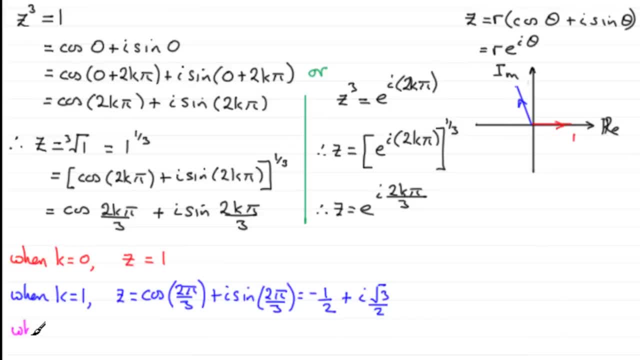 So what we need to do is take k to equal minus one. So when k equals minus one, Okay, what do we get? Well, we end up with z equaling the cosine of minus two thirds pi, which is in range. okay. 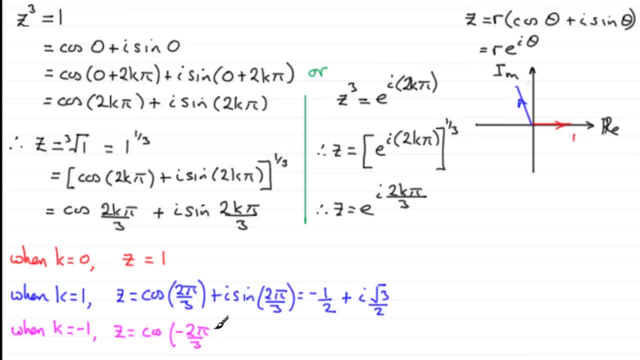 Minus two thirds pi And then plus i sine of minus two thirds pi, And when we work this one out you end up with minus a half and then minus. i root three over two. And if we were to plot this on the argon diagram, 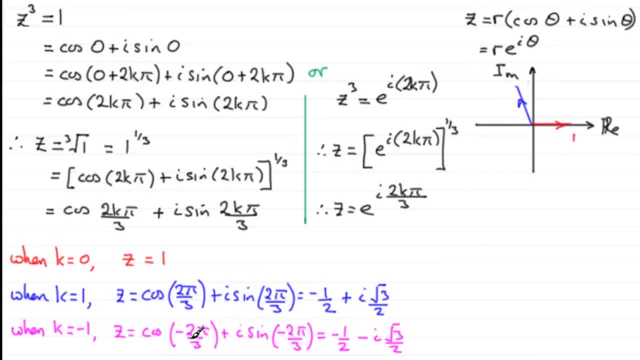 what we would find is that the arg is minus two thirds pi. Now, remember, this angle in here was two thirds pi. So it's just going to be turning in the clockwise direction. So it's just going to be turning in the clockwise direction for the same amount. 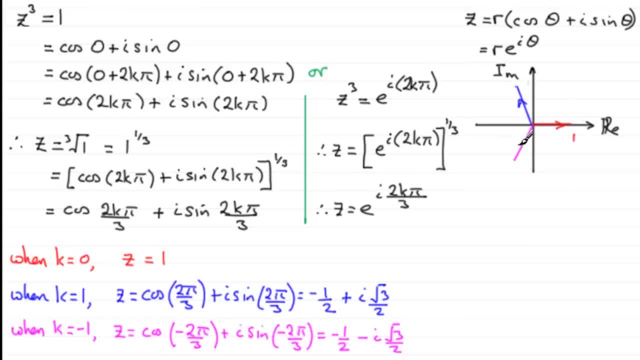 So it's going to look something like this. So it's going to look something like this. We'll just mark that on with an arrow like: so We'll just mark that on with an arrow like: so: Now, what we've got here is the three roots. 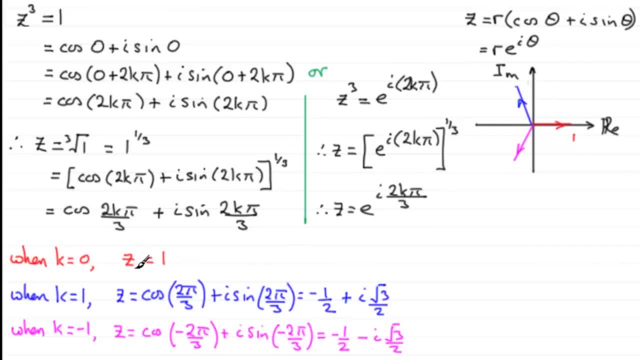 Now, what we've got here is the three roots. I might as well call them, say z1, z2, z1, z2, and z3.. And you'll notice that, And you'll notice that they're all equally spaced. 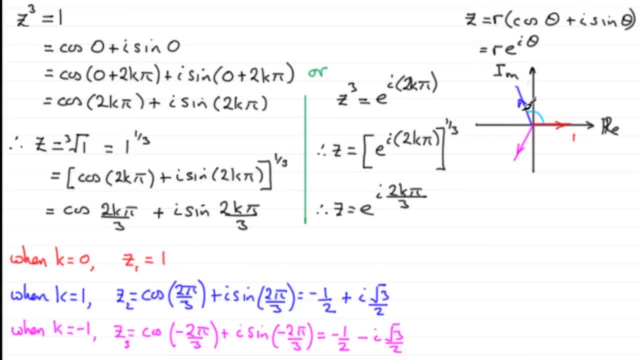 If I mark in this angle, this angle in here, this angle in here and this angle round here, each of those angles- let's just say we call them alpha- then alpha is equal to. then alpha is equal to two thirds pi radians. 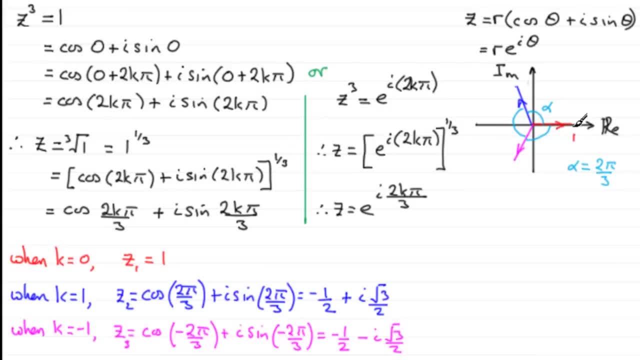 two thirds pi radians And also because they have exactly the same And also because they have exactly the same modulus: one unit. they lie on a circle of radius- one unit of radius, one unit. Let's put that in here, that we've got a circle. 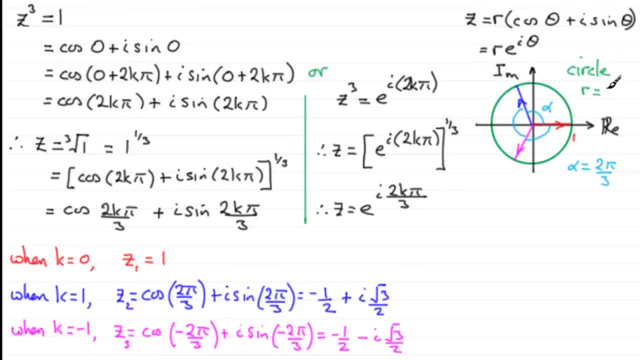 of radius. one unit of radius, one unit, So r equals one. Now we can write these solutions in then as z1. for this first one, Let's just write that in as z1.. And then the second solution we got here in blue was: 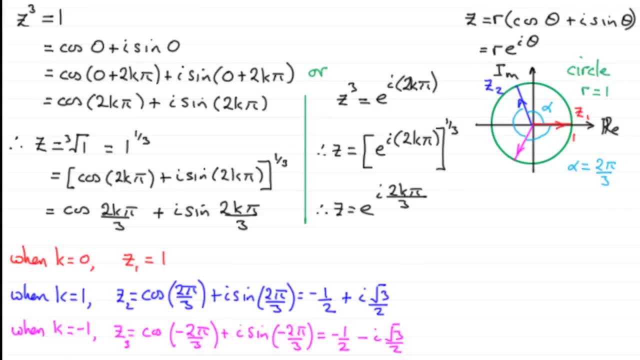 z2, say. And then the third solution: the root was z3.. Now, when I got these roots here, I took: k equals zero, k equals one, k equals minus one. I could have taken zero, one and two, but 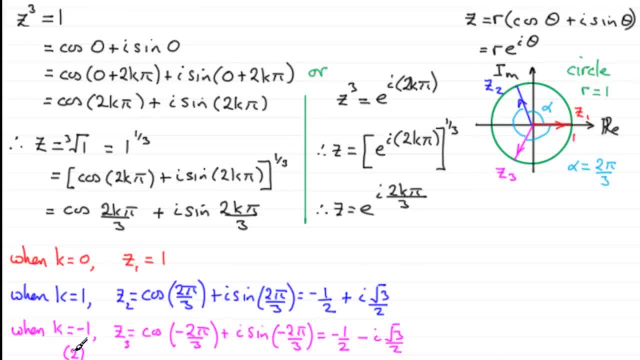 we don't tend to do this because, although it would have given us the same result- because if k equaled two, we would have had the cosine of four thirds pi plus i sine four thirds pi- That would have taken us to exactly. 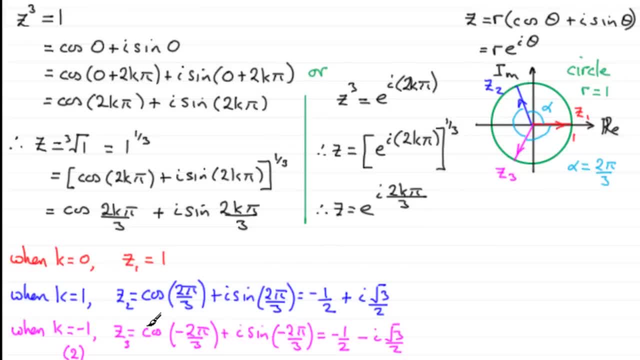 the same place as we've got here. But when we express a complex number in mod-arg form, the arg has to be greater than minus pi, but less than or equal to pi. So four thirds pi would have been out of range. 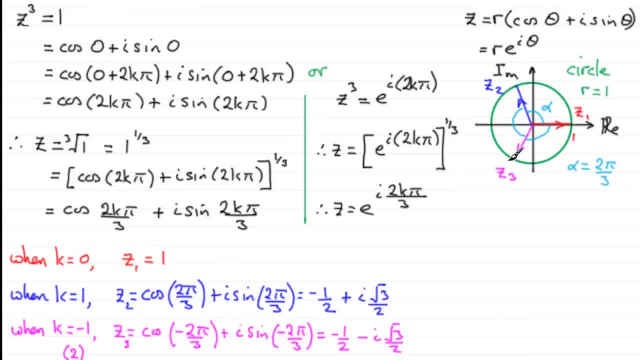 But, as I say, it would have given us exactly the same result, though. Now, if you were using the exponential form of representing the complex number z, then we would still take our values of k as being zero. It would have given us an arg of zero. 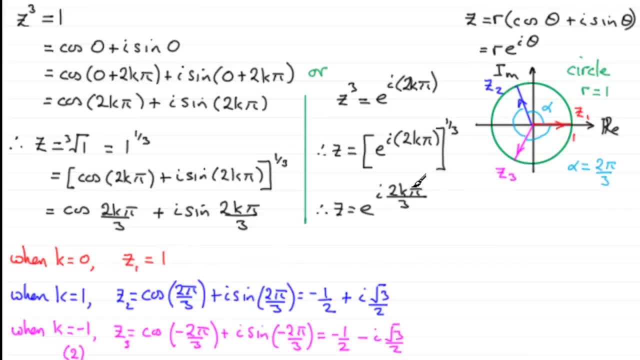 leading us to one. And then if k equaled one, we'd have had an arg of two thirds pi. It would have taken us to this point here, And it has a mod of one. And if we had taken k to be minus one, 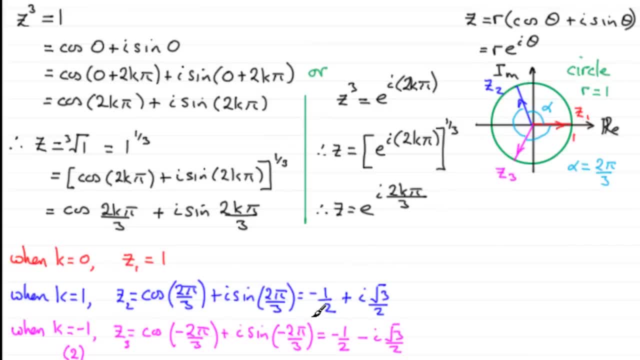 it would have given us an arg of minus two thirds pi, No different to what we've got here, and we would have gone round that way and the mod would have been one. So it's up to you again which system that you use. 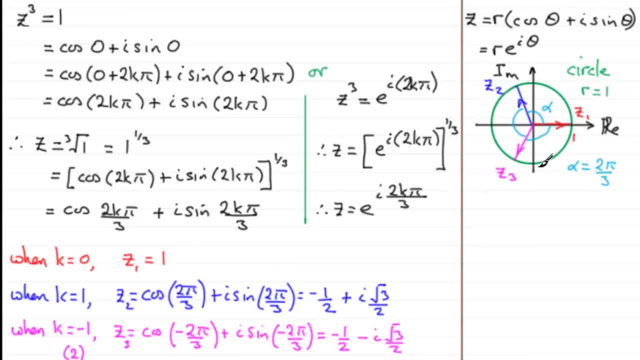 Now, some interesting results follow from this particular result. the nth roots of one, Remember, we're just looking at the cube roots of one, But if we take the first complex number, moving in an anti-clockwise sense away from the one, 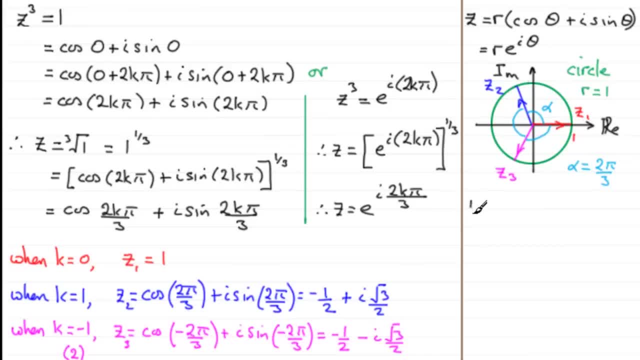 in this example it's z2, then if we let z2 equal, say omega, just write that in. then if we were to work out what z2 was squared, then you could either just square this result or you could use the result. 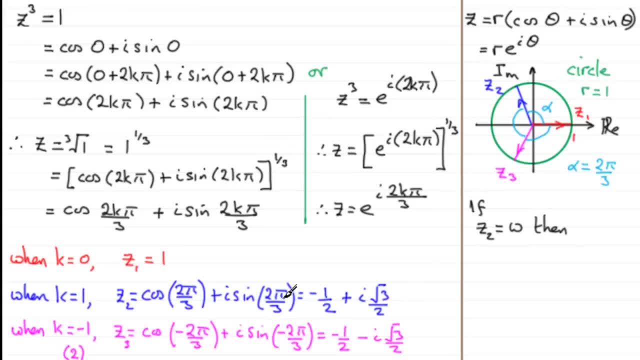 that if you're looking at the modulus of a complex number, this complex number multiplied by itself again, then all we do is we multiply the individual moduli together. So in other words, it'll just be one times one, which is one. 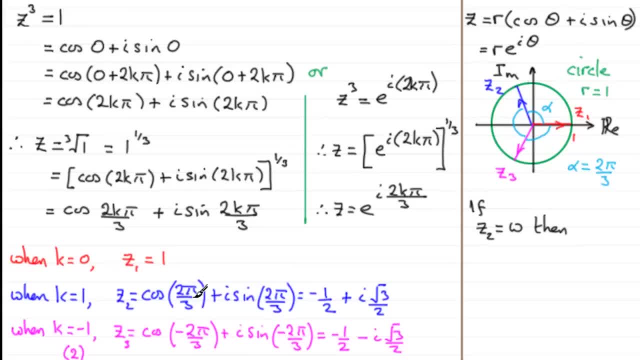 So we've got a complex number with a modulus of one, and remember that if you square a complex number you would add the args together. So you've got the cosine. well, the arg, I should say, is two-thirds pi. 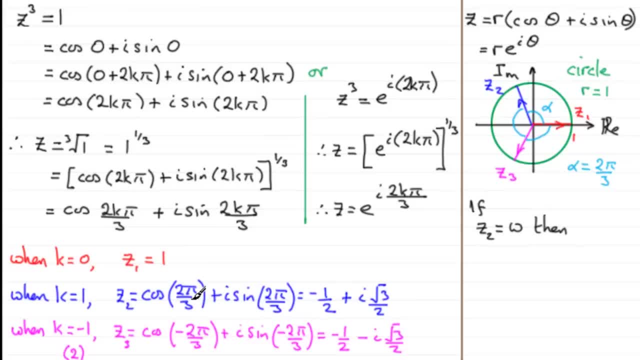 and if you were to double that, add it to itself again, you're going to get an arg of four-thirds pi, And an arg of four-thirds pi takes us round to here, which is the same as minus two-thirds pi. Can you see that? just by. 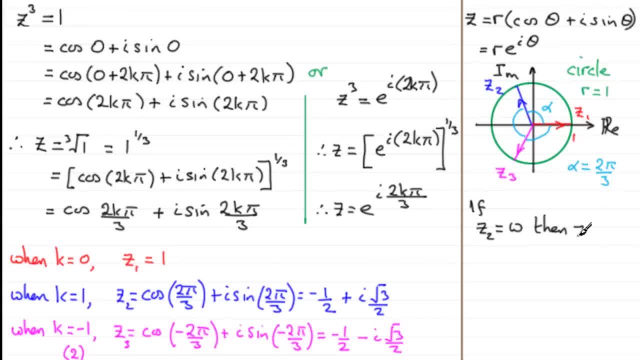 squaring z2, we're getting z3.. So z3 turns out to be omega squared or z2 squared. So I'll just highlight this result. okay, Just put a box round it And you'll find similar results like this when you 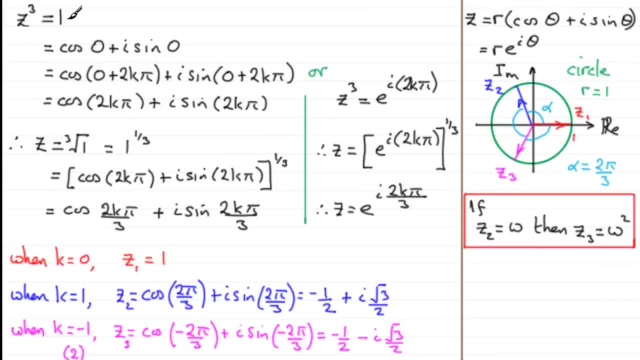 do further roots of one, okay. Now, another result that's worth looking at is the fact that z3 is the complex conjugate of z2, okay, So we get our results occurring, remember, in a complex conjugate pair. So, 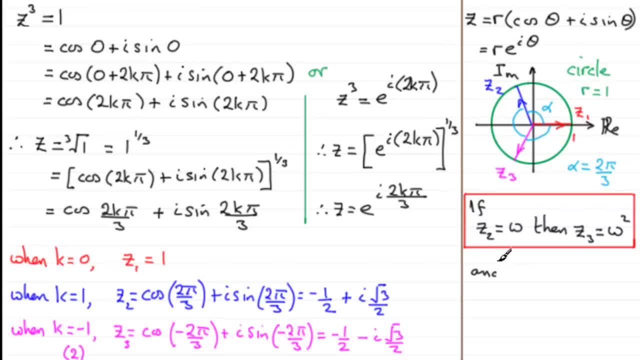 z2 was omega, so we've got that omega. if I take the complex conjugate of it, it equaled omega squared in this example. okay, So well worth mentioning that one. Now, another important fact that works with this is that 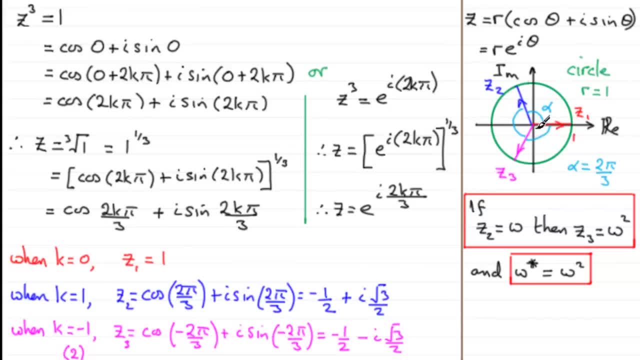 if we were to consider, say, these complex numbers that I've drawn as vectors, then if I was to draw z1, okay, let's just put this down here- z1, like that. okay, that's going to be one unit that way. 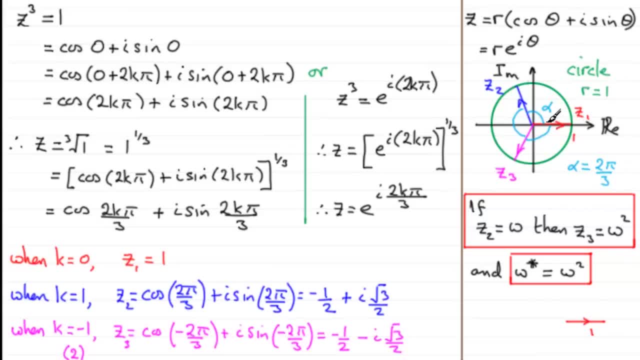 and follow it with z2, remember that's one unit and it's going to look something like that. Okay, We'll say that's omega now, and if I follow it with z3, which we've just seen is omega squared. 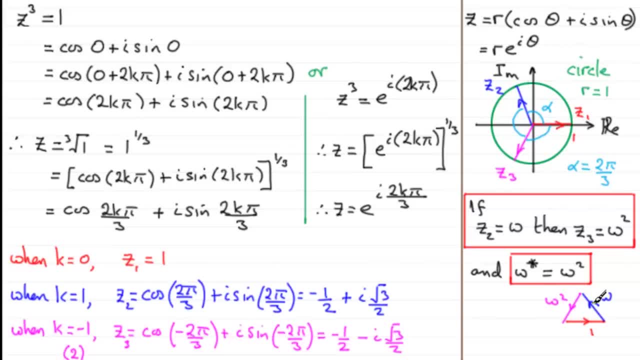 alright, it forms a closed triangle. okay, A closed polygon, if you like. Only the polygon here is a triangle. So what we've got is this result, just say: also okay. This result is that if we add these together, these complex numbers,